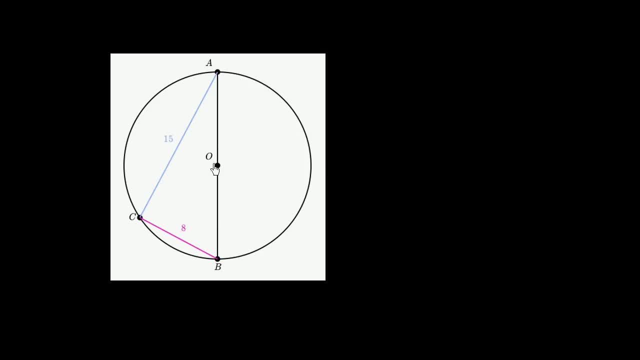 AB is definitely the A diameter of the circle. It's a straight line. It's going through the center of the circle. O is the center of the circle right over here, And so what do we know? Well, we could look at this angle right over here, angle C: 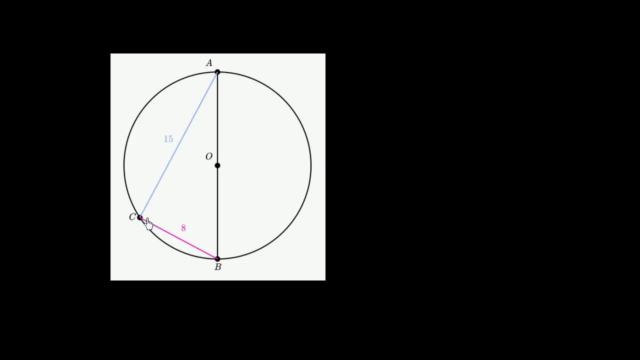 and think about it is an inscribed angle. And think about the arc that it intercepts. It intercepts this arc right over here. This arc is exactly half of the circle. This arc right over here is exactly half of the circle. Angle C is inscribed. 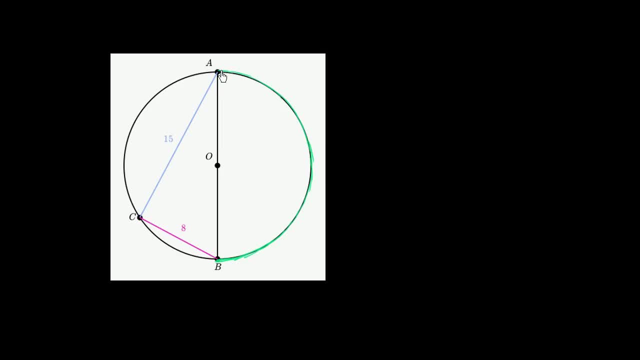 If you take these two sides, or the two sides of the angle, it intercepts at A and B And so it intercepts an arc, this green arc right over here. So the central angle right over here is 180 degrees. 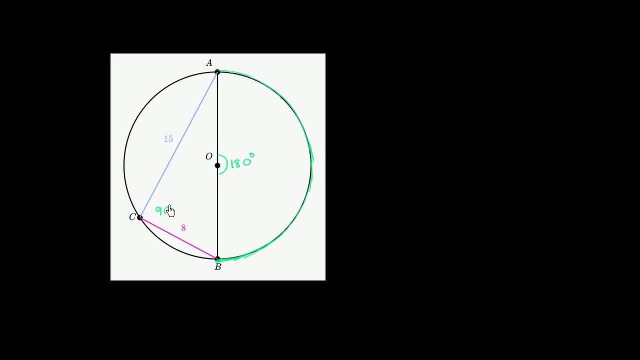 And the inscribed angle is going to be half of that. It's going to be 90 degrees Or another way of thinking about it. it's going to be a right angle And what that does for us is it tells us that triangle ACB. 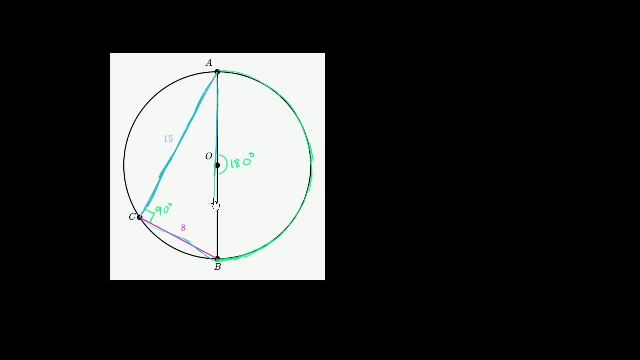 is a right triangle. This is a right triangle And the diameter is its hypotenuse. So we can just apply the Pythagorean theorem here: 15 squared, 15 squared plus 8 squared is going to be the length of side AB squared. 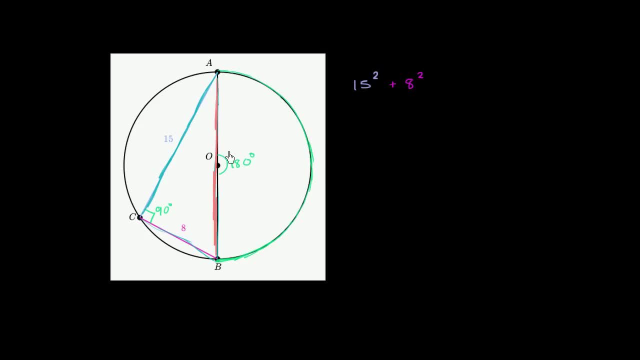 So let me just call this side right over here. Let me just call that x. That's going to be equal to x squared. So 15 squared, that's 225.. 8 squared is 64.. Plus 64. Is equal to x squared. 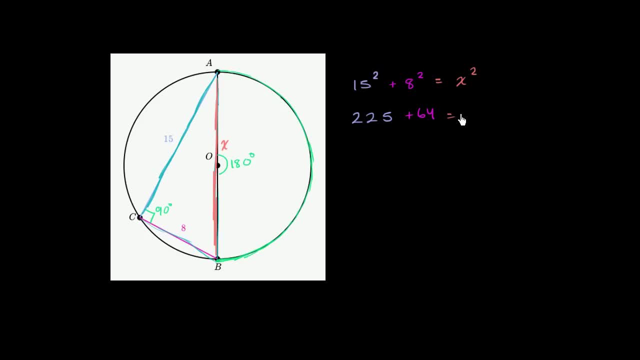 I want to do that in green. Is equal to x squared. 225 plus 64 is 289.. Is equal to x squared, And then 289 is 17 squared And you could try out a few numbers if you're unsure about that. 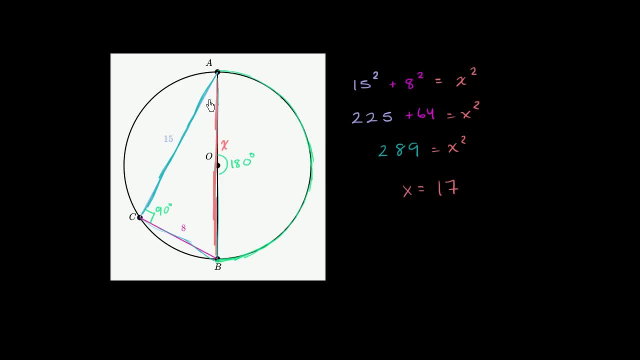 So x is equal to 17.. So the diameter of the circle, The circle right over here, is 17..